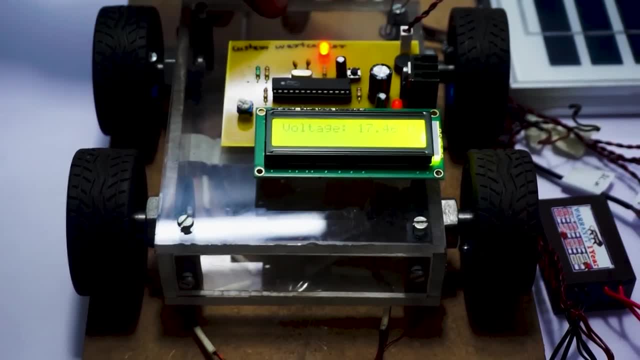 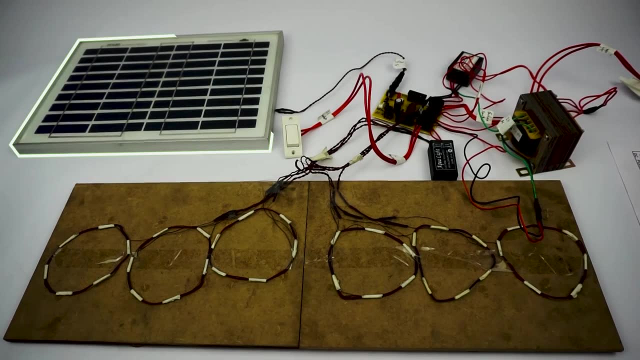 charging and it is charged continuously as it goes over the road. so these coils are connected to a transformer which is used to power them. how basically the system works in the solar panel you can, as you can see here, it used to charge the battery using charge controllers, so the charge from the battery is 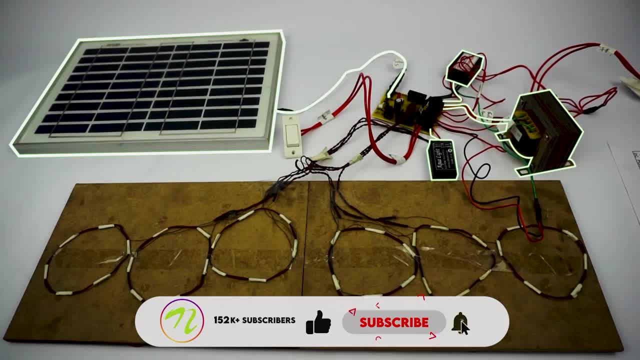 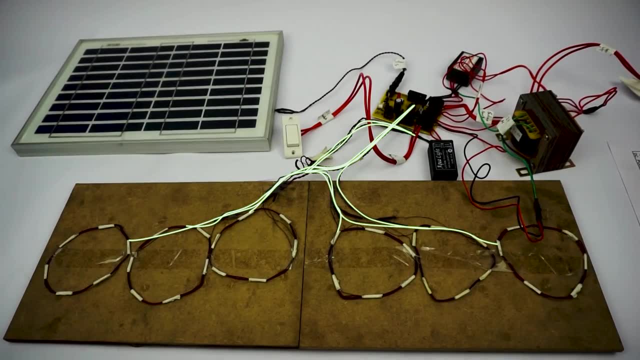 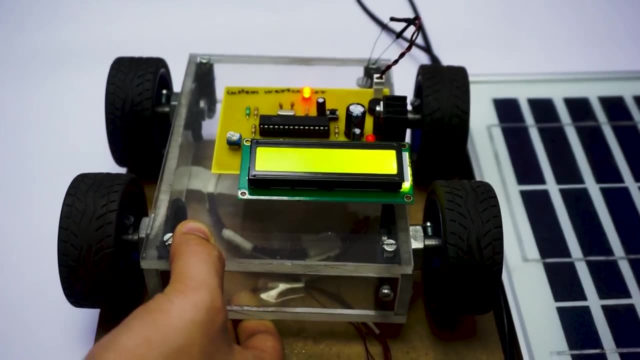 converted to AC power using the transformer, because for wireless transmission we need the power to be AC power. and after the power is transmitted from the coils on the road, it is received by the coil underneath the vehicle and this perceived power again converted into DC so that it can be used. 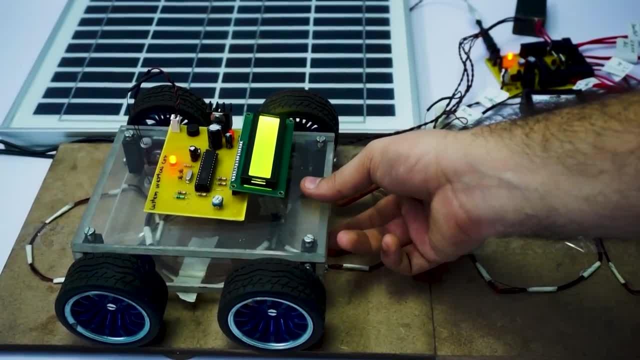 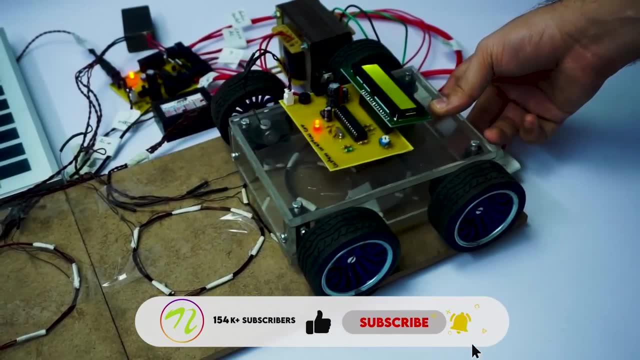 to charge the vehicle battery. so now let's move the vehicle over the track and, as you can see, as it moves over the road, the power is transferred wirelessly to the solar panel circuit and, as you can see, the box of the vehicle is made to be transparent and 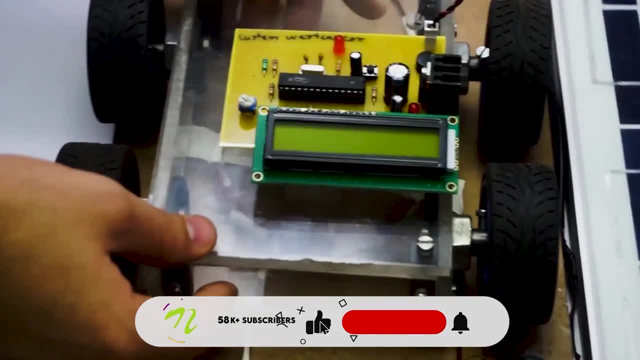 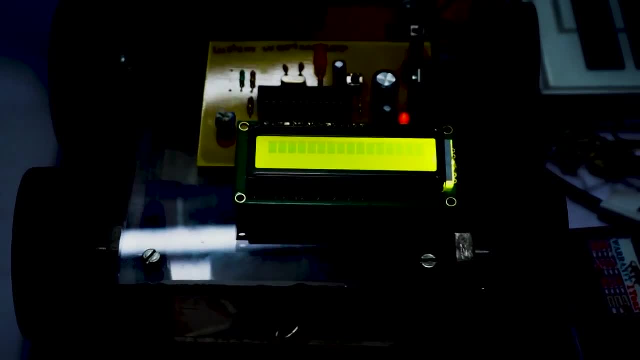 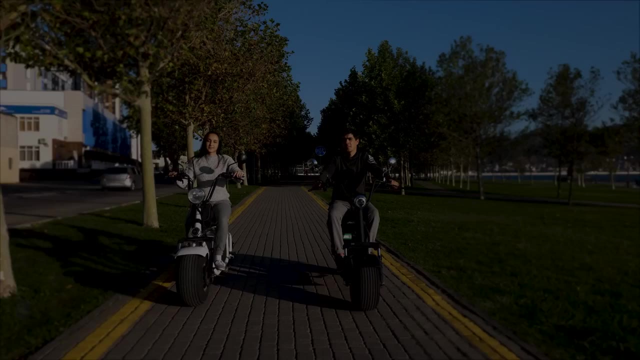 the coil that is mounted inside the vehicle is used to power vehicle circuit and also show the voltage generator. so here we can see the voltage that is generated, received at the vehicle and as it moves over the road. so this is how the system works. e-bike speed controller system. electric bikes are gradually 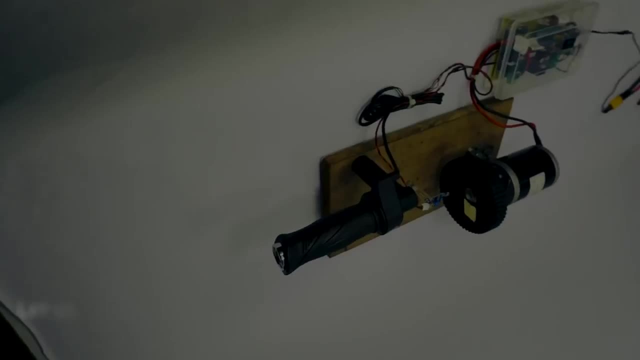 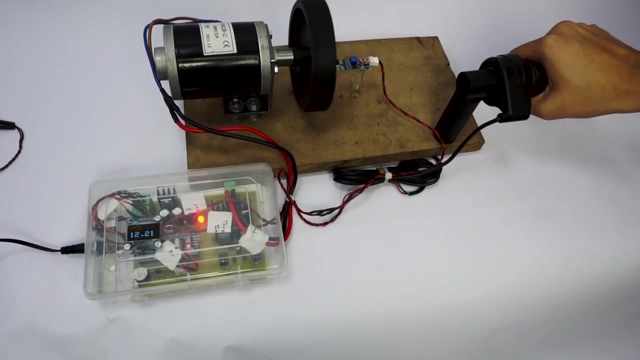 taking over the fuel based bikes, as it is more environment friendly. let us look at this new system which controls the speed of an e-bike. as for its throttle to the throttle acts like a potentiometer, which is the input of which is fed to the HTM32 microcontroller and, based on that, the 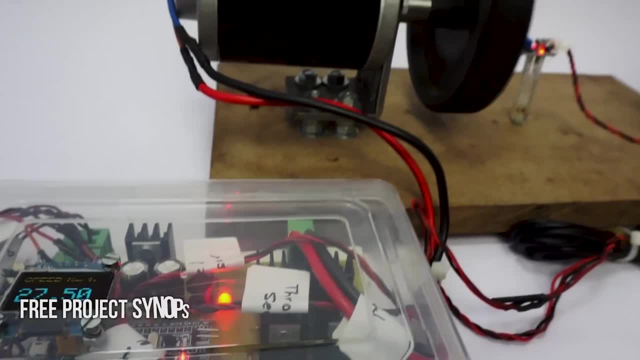 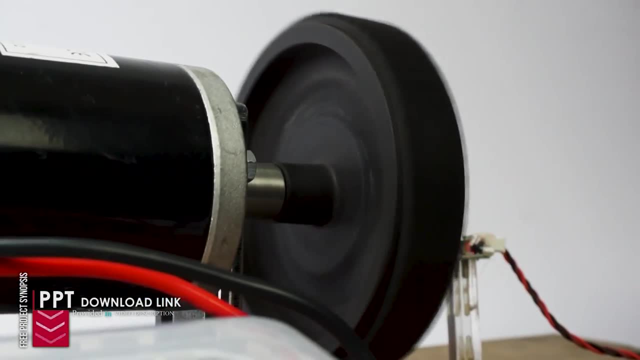 controller will operate the DC motor. the controller will increase the speed and as the speed increases, the wheel speed increases. and we have a sensor here. it is a IR based sensor which is used to measure the speed. the measured speed is then displayed on the OLED display using the HTM32 controller. 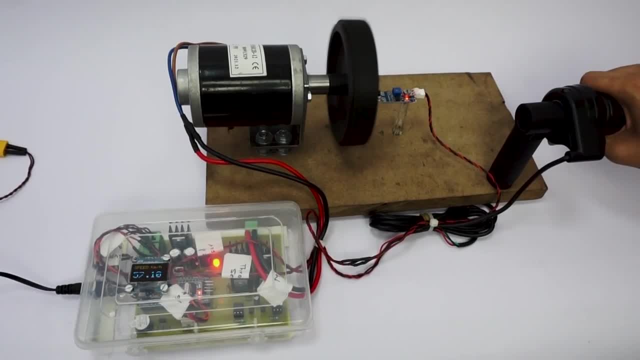 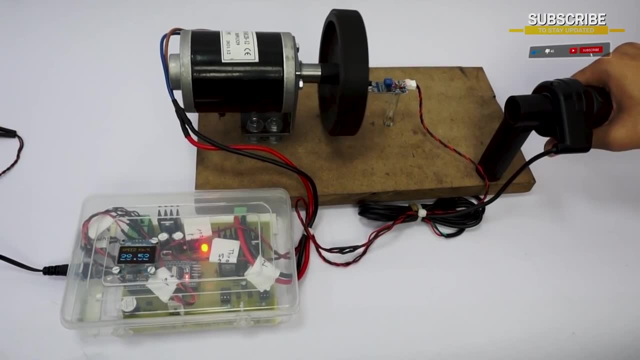 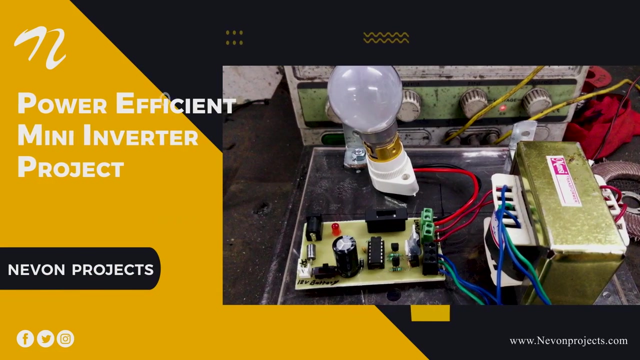 controller. So let's increase the throttle. We have increased it to the maximum and now let's decrease it gradually. So, as you can see, as we decrease the throttle, the speed keeps on decreasing until it reaches zero. Power Efficient Mini Inverter- Project Inverters are widely used in domestic as well. 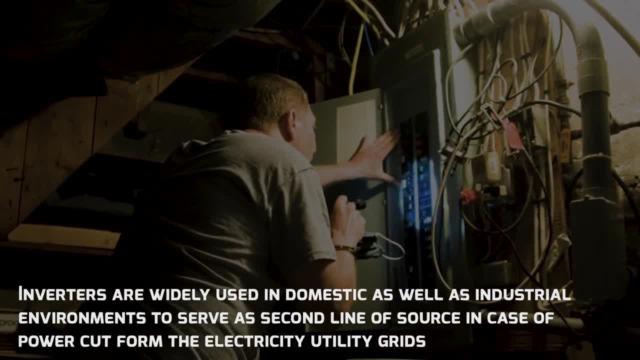 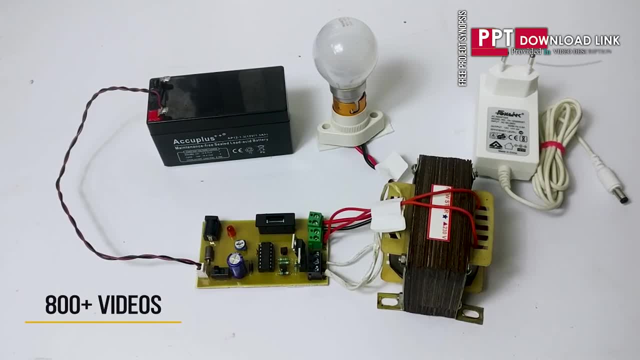 as industrial environments to serve as a second line of source in case of power cut from the electricity utility grids. Let us check out this mini inverter project. Let's assume that we are facing a power failure and the inverter is off, So the load remains. 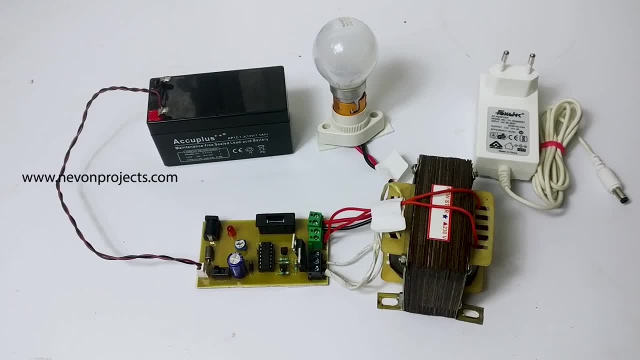 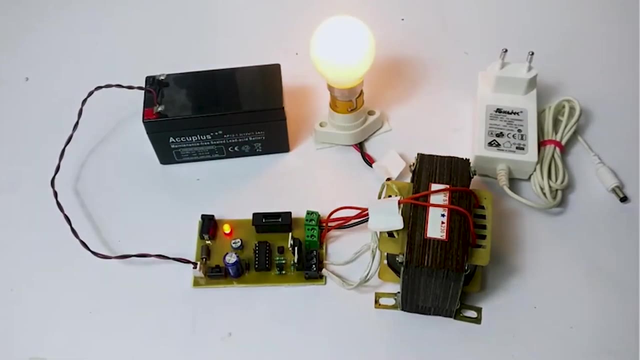 off. Now let's turn on the inverter. As you can see, the inverter converts DC to AC to power the load. Also, there is provision for charging the battery. The user simply needs to plug in the adapter here for charging the battery. 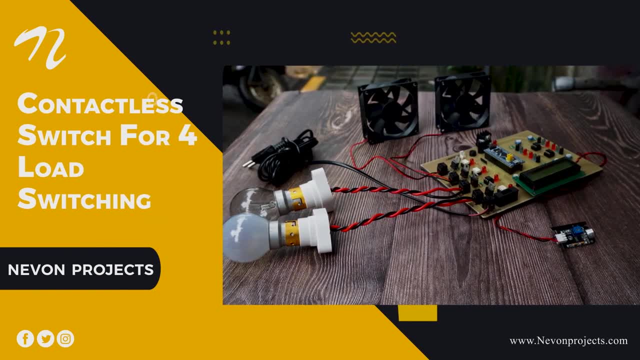 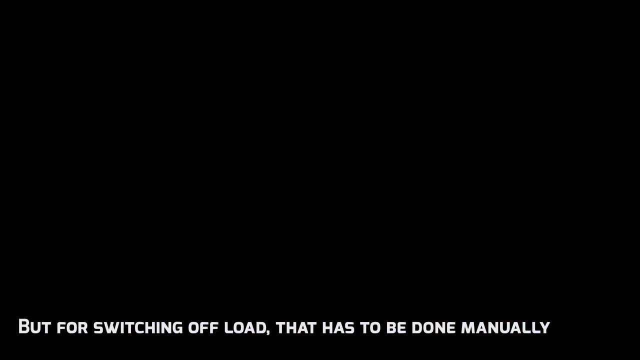 Contactless Switch for 4 Load Switching. Home automation has made life easy. Now everything is contactless, But for switching off the load. that has to be done manually. But with this new system we can switch off the load without any contact. 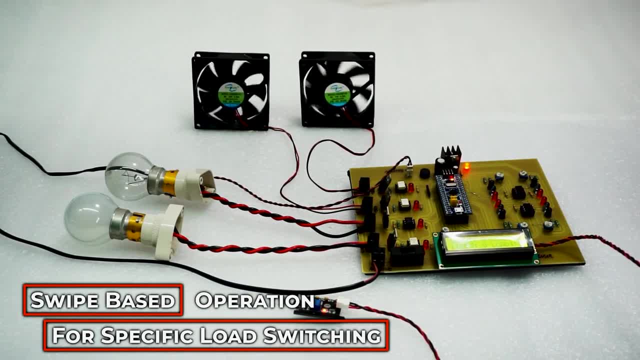 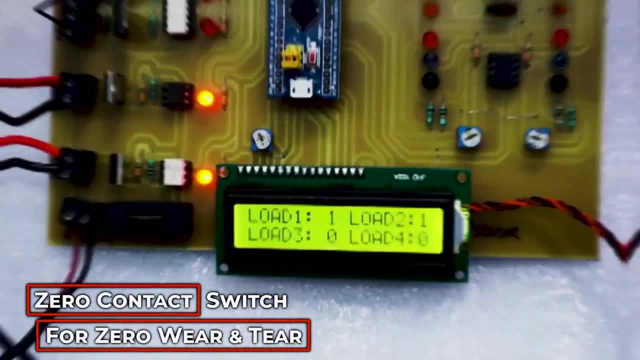 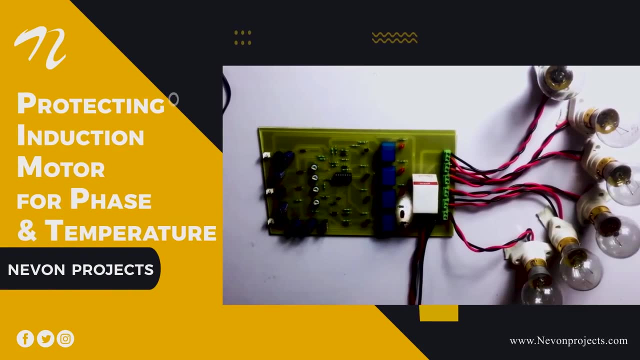 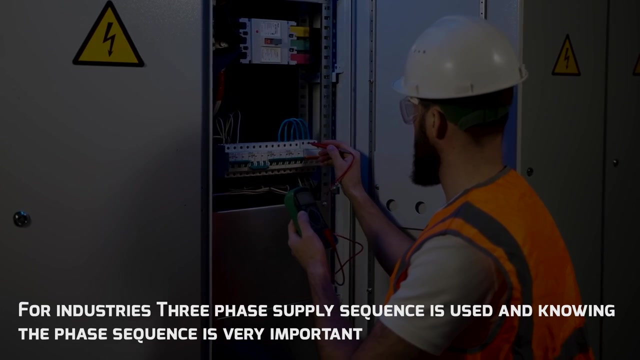 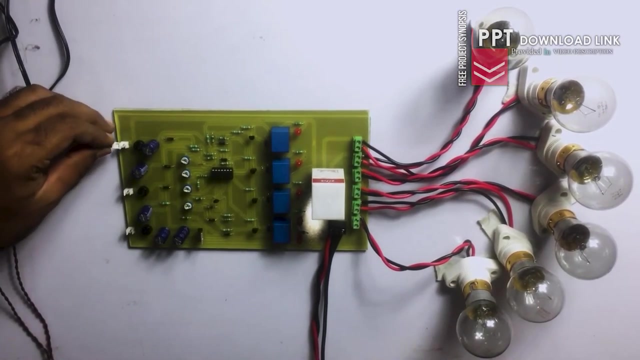 Protecting Induction Motor for Phase and Temperature. For industries, three-phase supply sequence is used and knowing the phase sequence is very important. So let us look at this system of protecting induction motor for phase and temperature. These are three transformer connections that we have shown for phase. So this was phase. 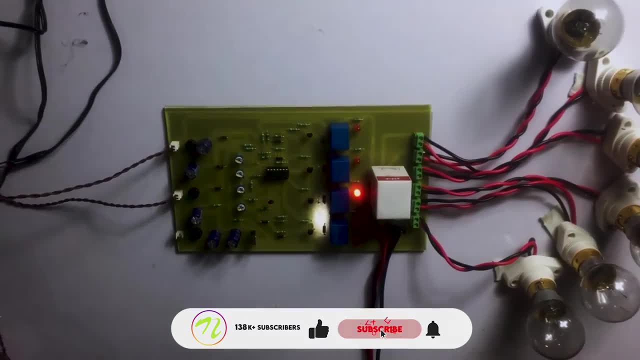 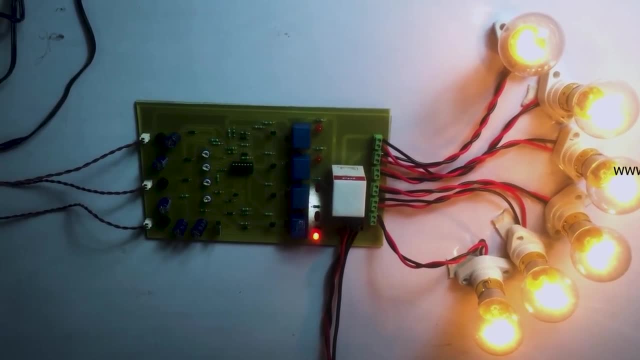 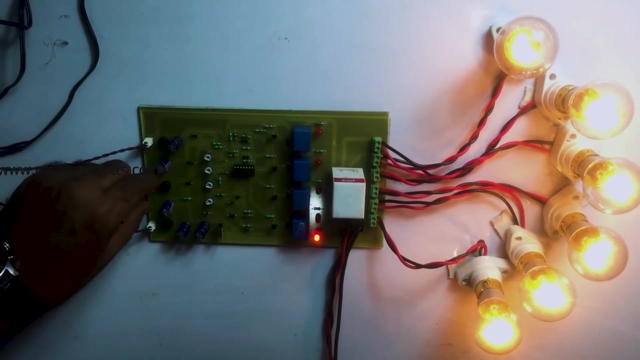 1.. This is phase 2. And this is phase 3.. So all the loads are off on. That means the induction motor is basically will now turn on And suppose if any one of the phase goes out, it is denoted. 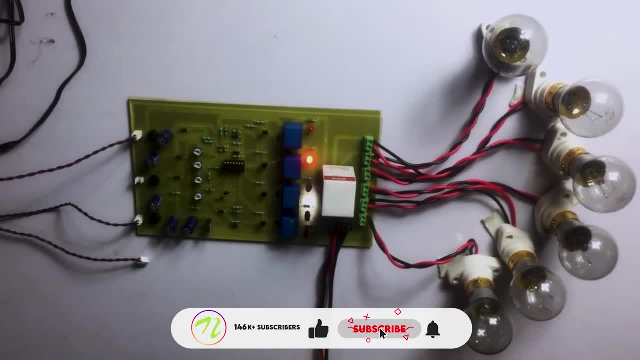 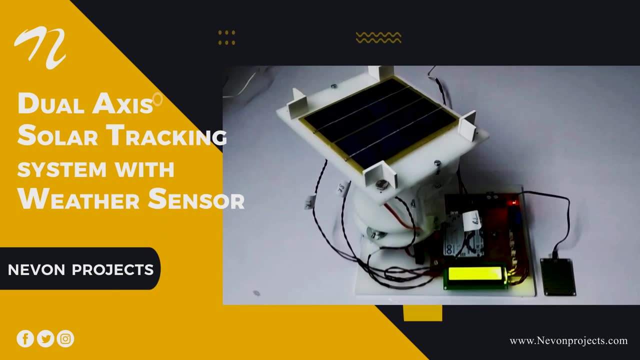 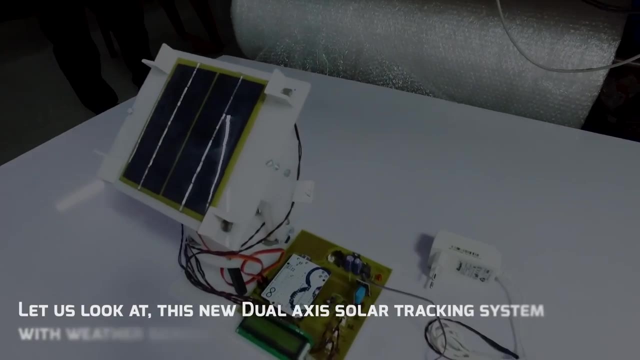 by the blinking LED Which shows that phase 2 is out And therefore the induction motor has turned off. Dual-Axis Solar Tracking System with Weather Sensor. Solar energy is renewable and will never run out, unlike other sources of energy. Let us look at this new dual-axis solar tracking system with weather sensor. This system can